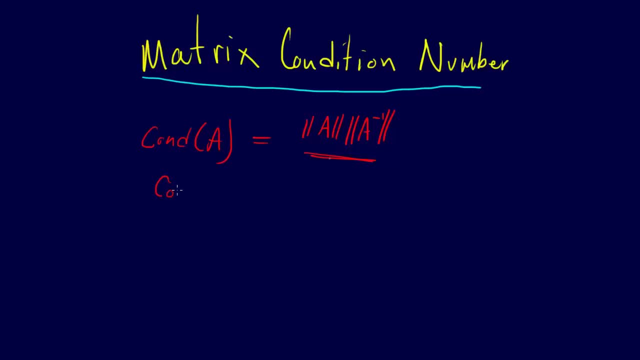 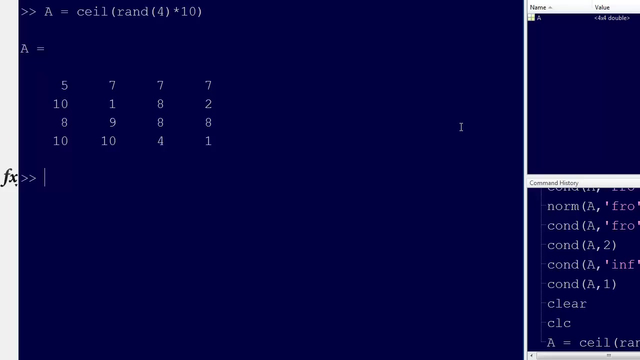 Now it's important to note that the condition number depends on the norm used. So one way of showing this is: let me just flip over to MATLAB and say: let me create a matrix A, And so there's my matrix A And I can do the condition number of A using the one norm. 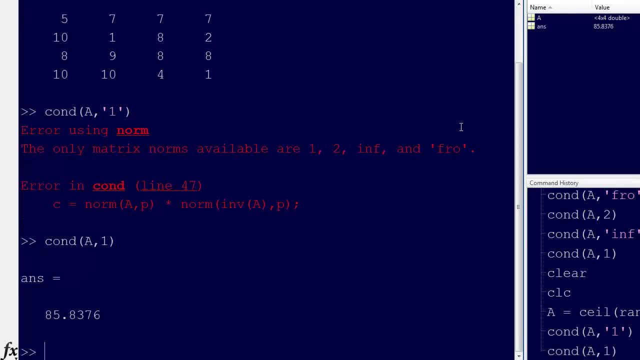 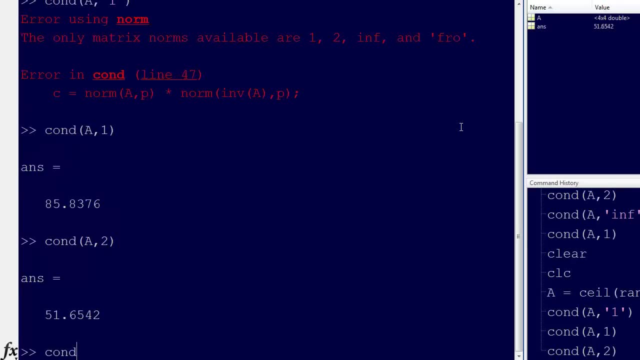 Whoops using the one norm. Okay, or I could do the condition number of A using the two norm, Or I could do the condition number of A using the Frobenius norm, Or the condition number of A using the The infinity norm. 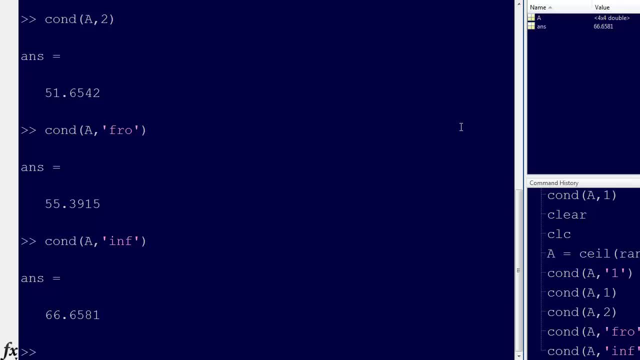 And you see we get slightly different answers. But for any given norm we could say the condition number of A, let's say using the Frobenius norm, And we could say the norm of A, the Frobenius norm of A. okay, 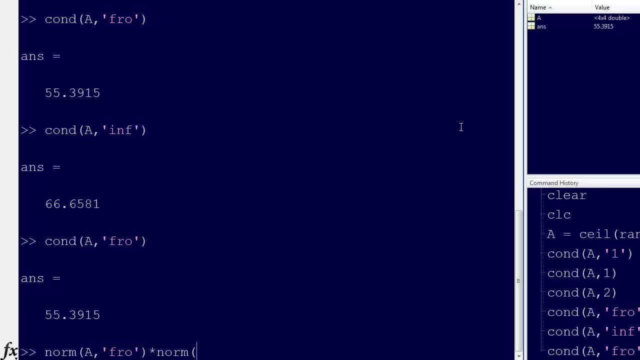 times the Frobenius norm, Let's say the Frobenius norm of A inverse, so inverse of A Frobenius, And we'll see that it comes out to the exact same thing. So, as just putting it in this way, that's exactly what this syntax is, just simply computing this. 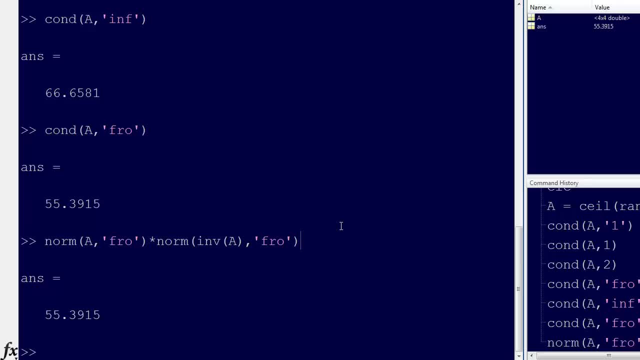 And so you see the condition numbers. they do vary a little Depending on the norm, But they're going to be a little bit tighter with some norms, a little bit looser with other norms, But they're going to give you an idea of the condition of the system. 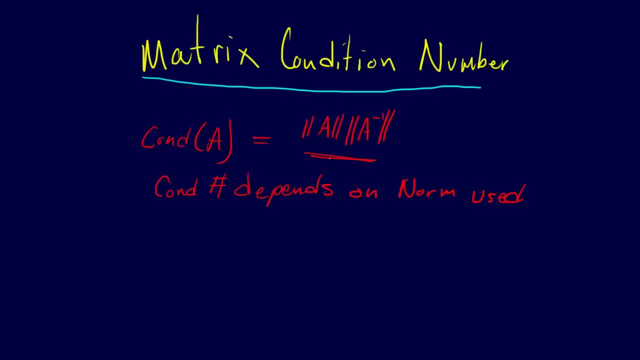 And the larger the condition number, the worse the condition of the system is. So large condition number is bad, okay, And by large condition number, Just several orders of magnitude, is bad.